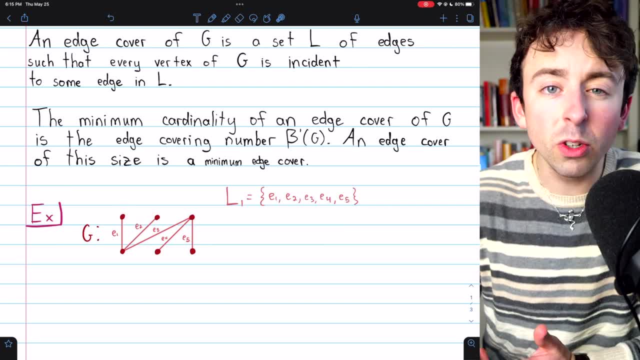 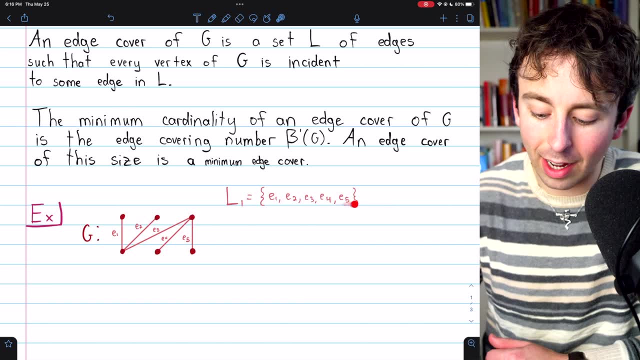 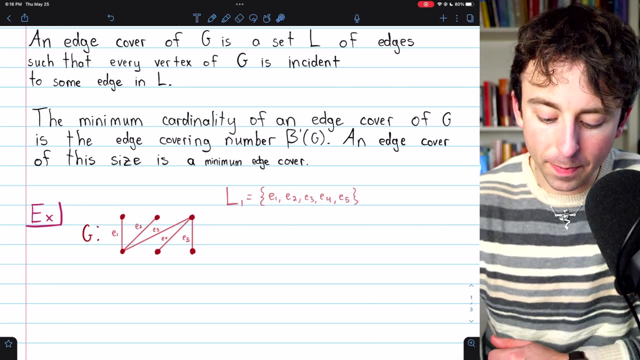 E1. So the vertex is incident to at least one edge in the cover. Similarly, this vertex here is incident to at least one edge in the cover. It happens to be incident to three edges actually: E1, E2, and E3. This vertex over here is covered by the edge E5.. This vertex here 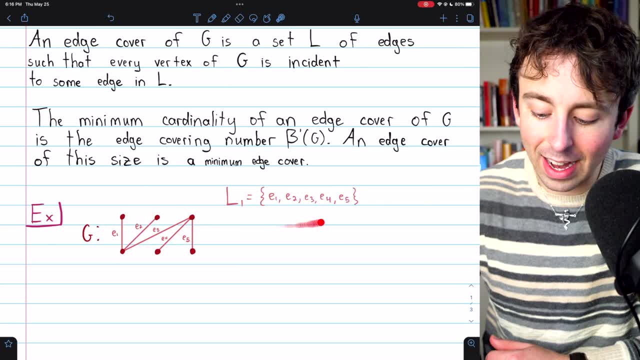 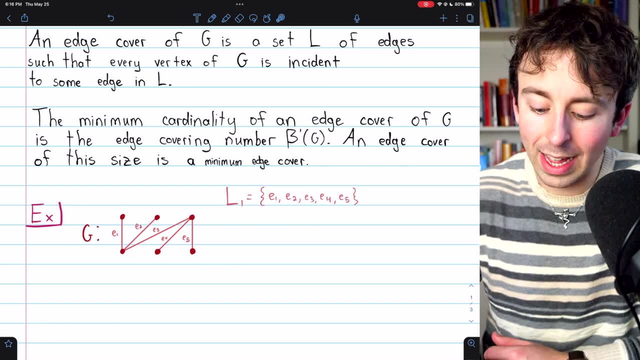 is covered by E4, and so on. This is an edge cover of the graph. Every vertex of G is covered by some edge, maybe one, maybe more than one in this cover L1.. In this case, L1 is not a minimum. 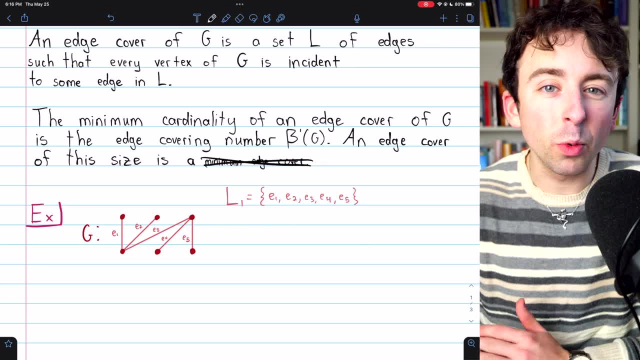 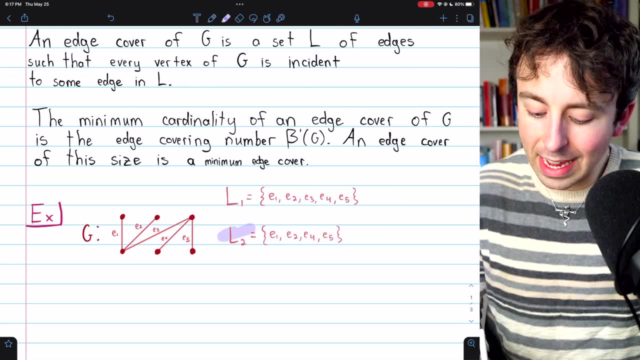 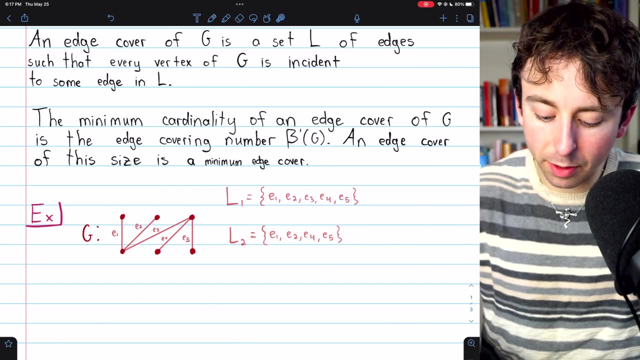 edge cover. We've included every single edge of the graph which is not necessary to cover this particular graph. Can you think of a smaller edge cover? Well, here's one. We don't actually know where the edge of an edge will be covered. at the moment We don't know which two edges. 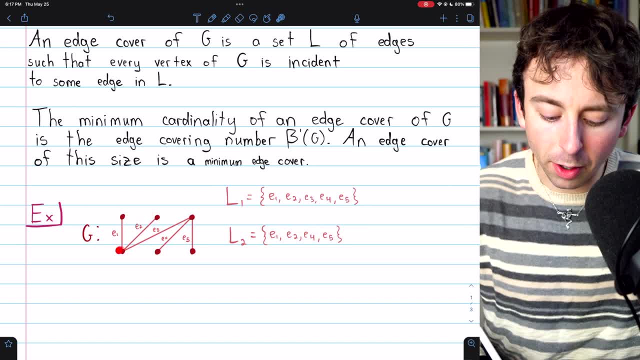 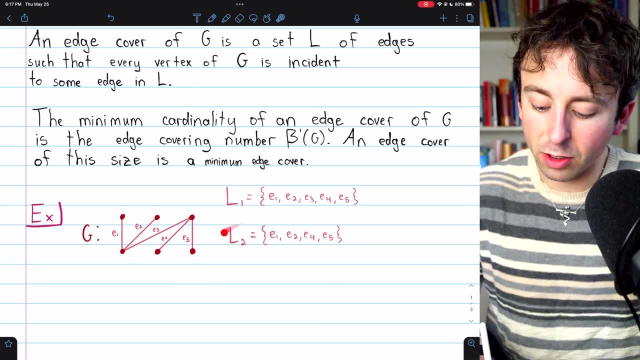 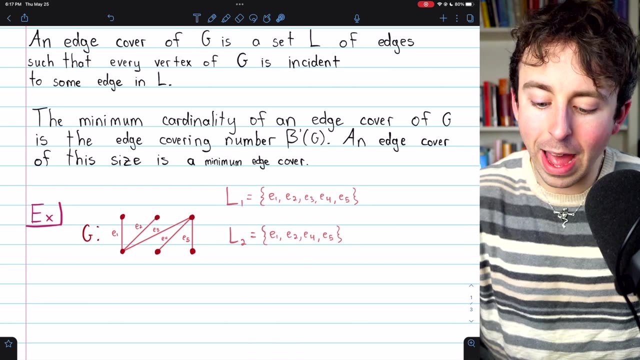 are simply covered either. You might not misunderstand that For word of opinion certainly. However, think of an edge cover E1 together. I don't know, None of us can think of that. The大家 surrounded that first line as an ellipse out to the right of the line. 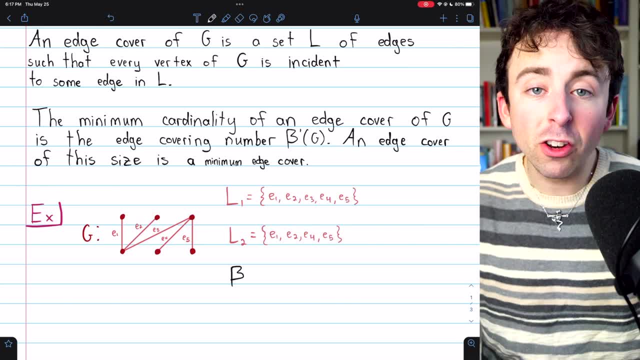 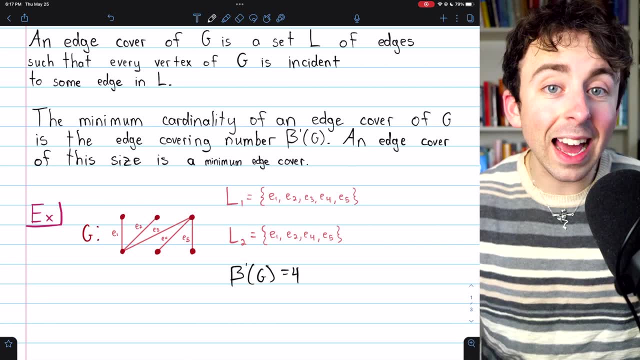 14 at the end of the line, We could better guess. covering number of G. written like this: beta prime of G is equal to 4, because that's the cardinality of a minimum edge cover of the graph. In this case it's actually quite easy to see that. 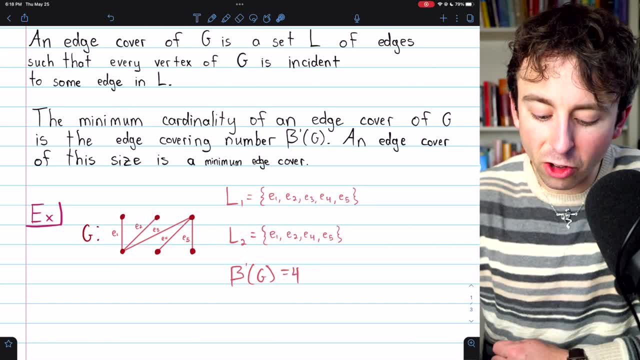 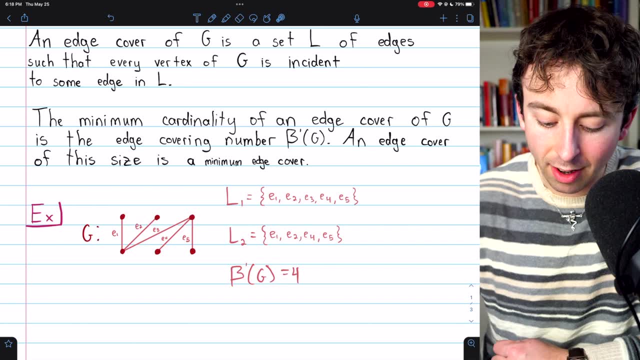 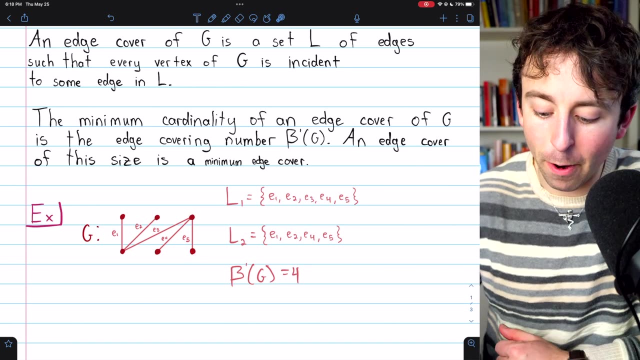 this is a minimum edge cover because for sure we need the edge E1 to cover that vertex. There's no other option. Similarly, we need E2 to cover that vertex, we need E4 to cover that vertex and we need E5 to cover this vertex. So it's immediately apparent that all of these edges are necessary. 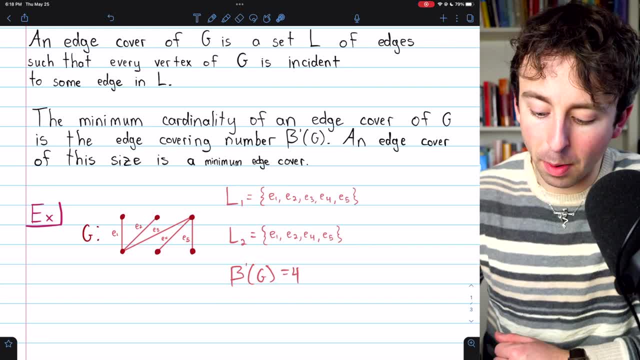 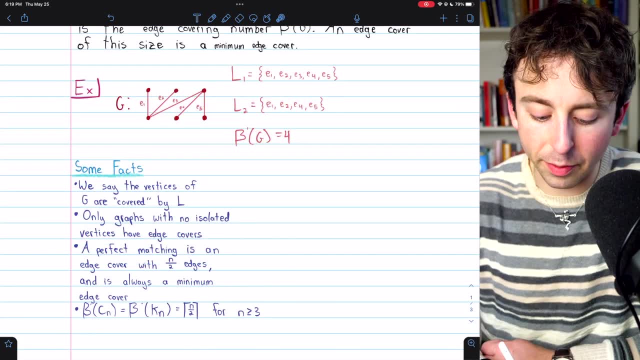 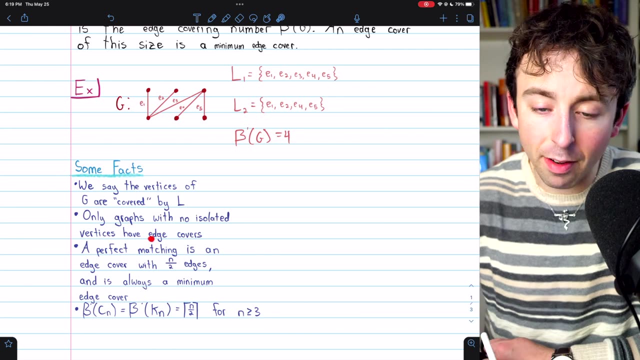 and we see in fact they are sufficient. So this is a minimum edge cover. the edge covering number of this graph is 4.. Here are some basic facts about edge covers. We say that the vertices of a graph are covered by its edge cover. Only graphs with no isolated vertices have edge covers. So 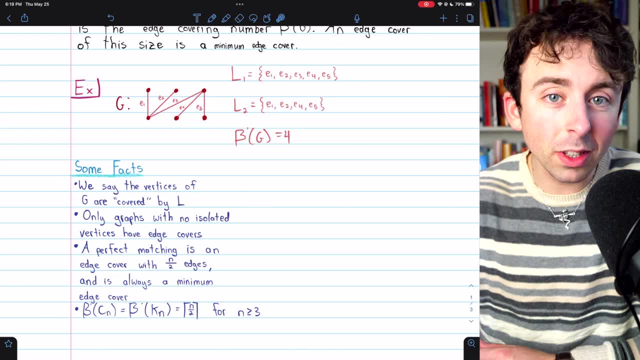 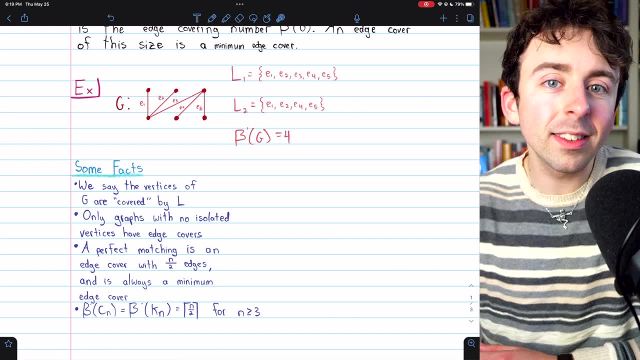 earlier I said, if you just take all edges of a graph, usually that will be an edge cover. the case where it wouldn't be is if the graph has isolated vertices. If a graph has isolated vertices, you could take all of its edges. you're still not going to be able to cover that isolated. 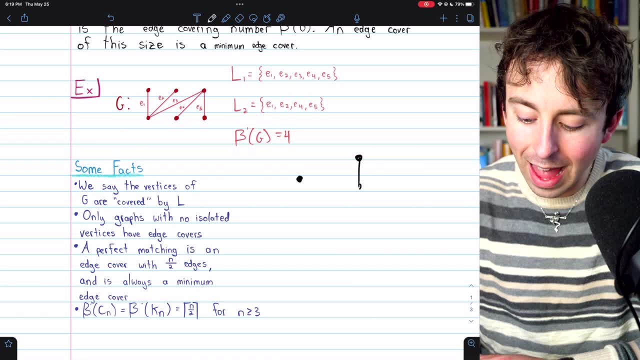 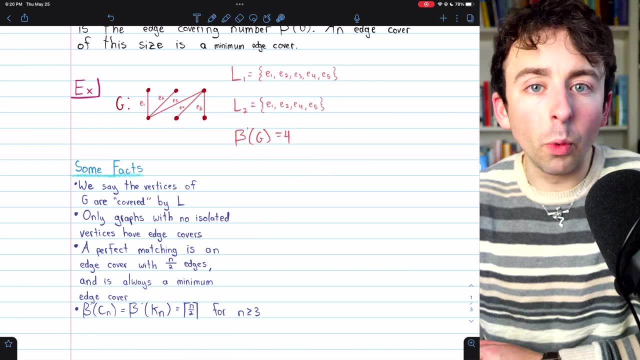 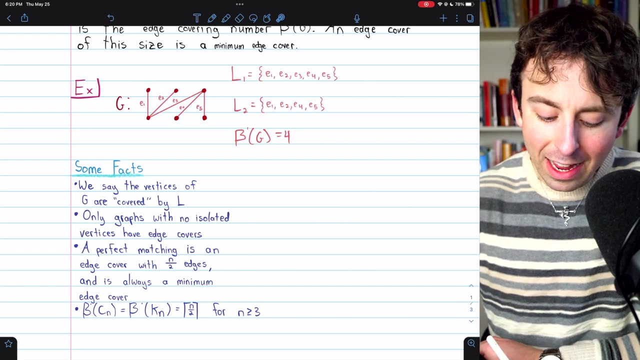 vertex. So a graph like this, for example, has no edge cover. There just is not a way to cover that isolated vertex. Now you may recall what a matching in a graph is- Link in the description to my lesson introducing that topic. A perfect matching is an edge cover with. 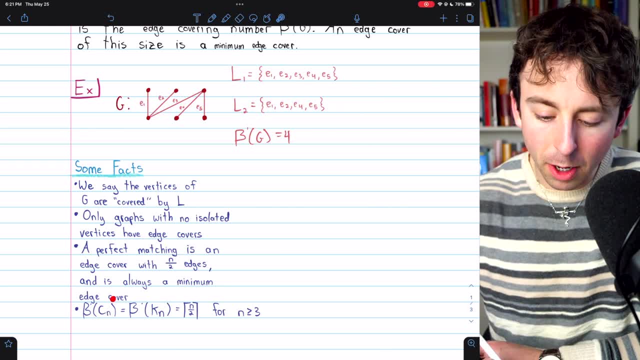 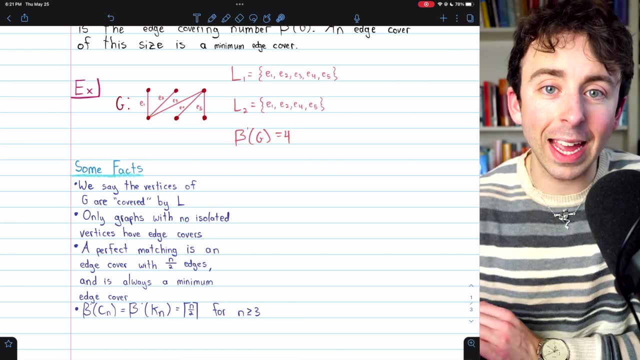 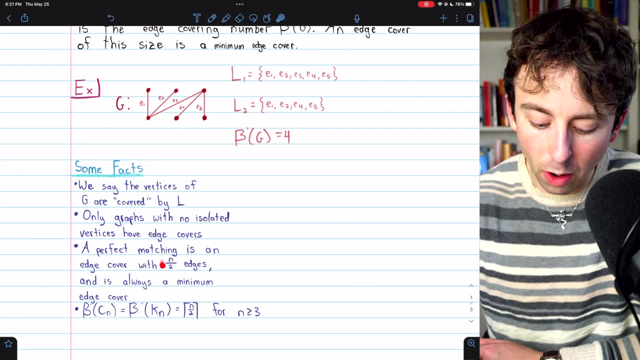 n over two edges, and this is always a minimum edge cover. That's because each edge could at most cover two new vertices that aren't covered by any other edge in your edge cover. So the most efficient possible edge cover would have n over two edges. Each edge is covering two distinct. 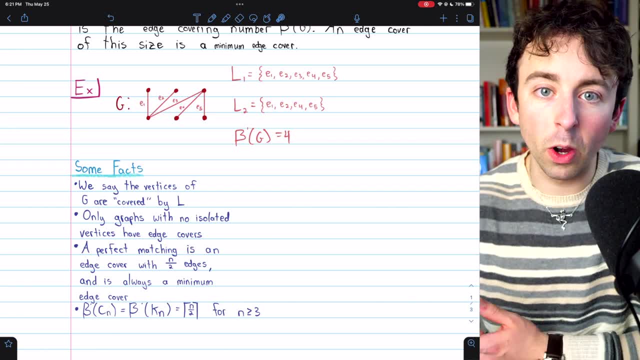 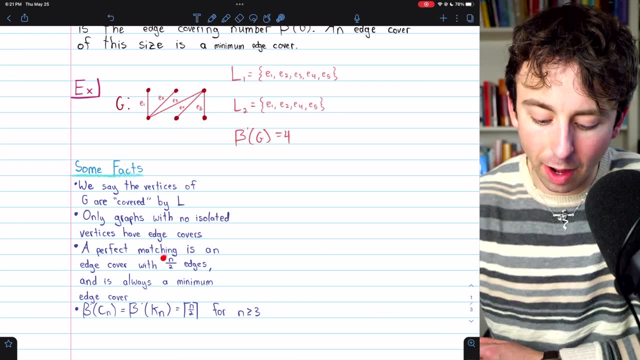 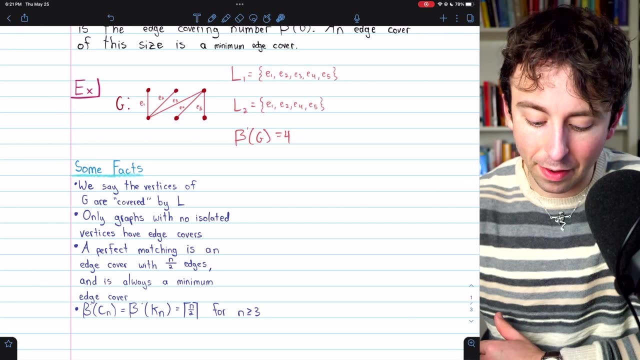 vertices unique from any other edge, and so in total it would take n over two edges at least to cover all vertices in a graph. So if you have an edge cover with that minimum n over two edges, that will always be a minimum edge cover. Of course, not every graph has such an edge cover And it's also called 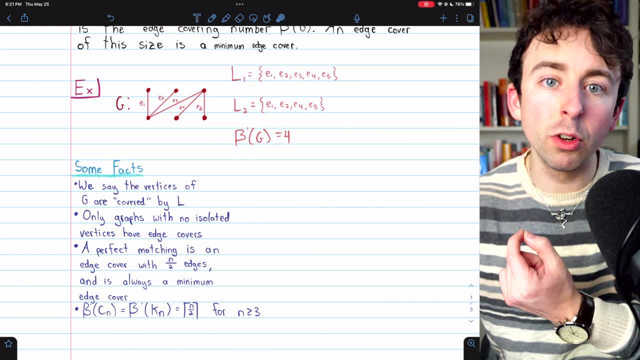 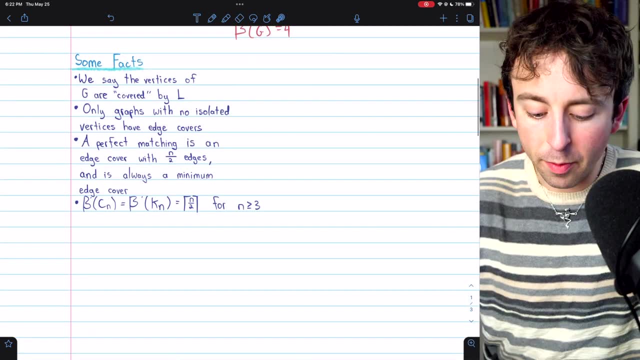 a perfect matching because each edge matches two vertices. so you have perfectly matched the vertices in a graph with this sort of edge cover. Finally, some edge covering numbers for two common families of graphs. The edge covering number of the cycle graph with n. 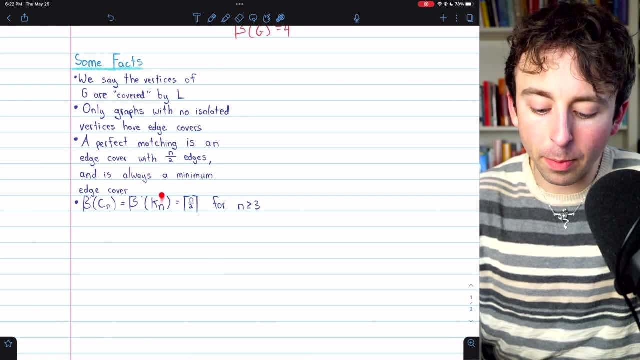 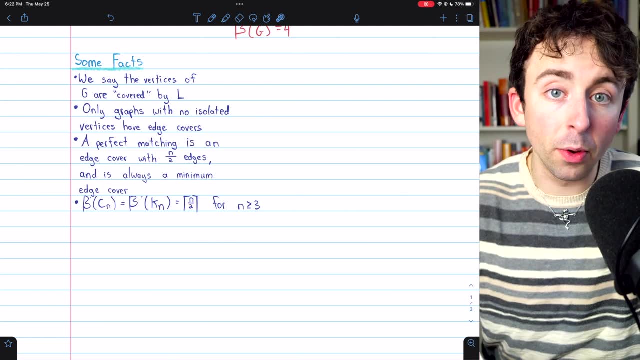 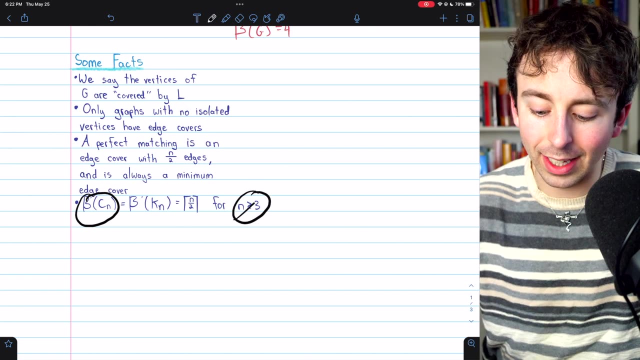 vertices is actually the same as the edge covering number of the complete graph. on n vertices. They're both just n over two rounded up, if it's not an integer, although this only holds for n at least three. Of course, the cycle graph cn is not defined when n is less than. 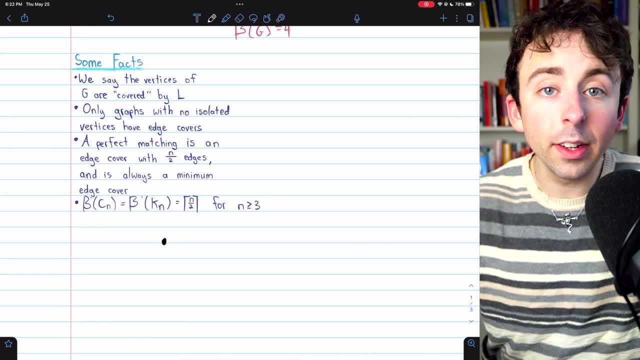 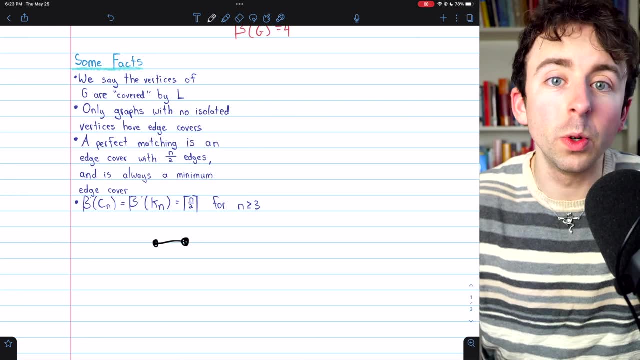 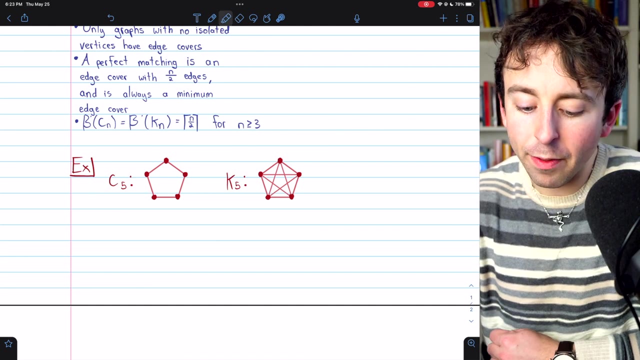 three and as far as complete graphs go, k1 does not have an edge cover and for k2 the formula does apply. The edge covering number is two divided by two, which is one. Here's one final example. Here's an example with c5 and k5.. Looking at the cycle graph, with five vertices again,